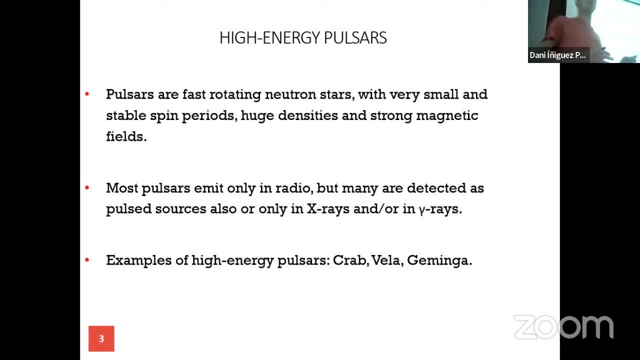 As you probably know, cultures are far-rotating from stars, which are compact objects in very small and stable periods with huge densities and very strong magnetic fields- the strongest magnetic fields we know in the universe. At the present moment, almost 3,000 cultures have been detected. We know almost 3,000 cultures. 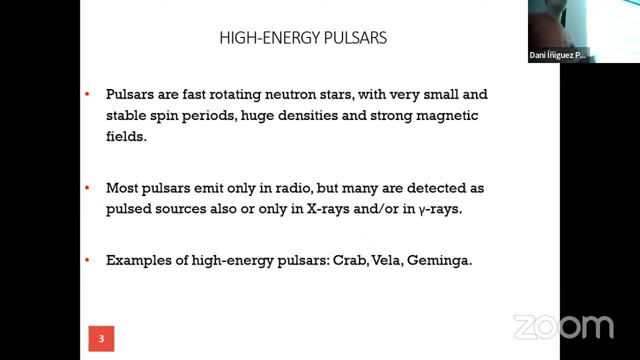 But some of them, around 200, has also detected grahamet freq radiation. These factors are so called gamma ray pulsar, mostly detected by radio microscope. Other than those around 40 of them haveixoemit not thermal X-ray simulations. 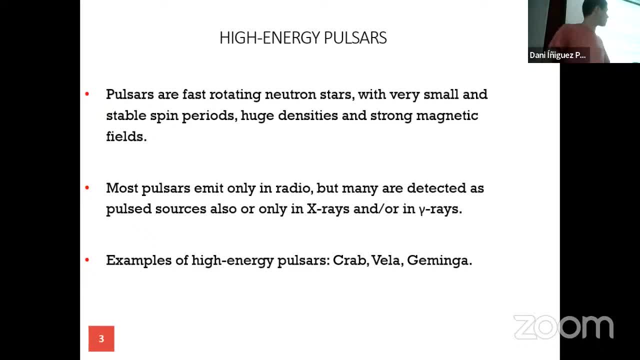 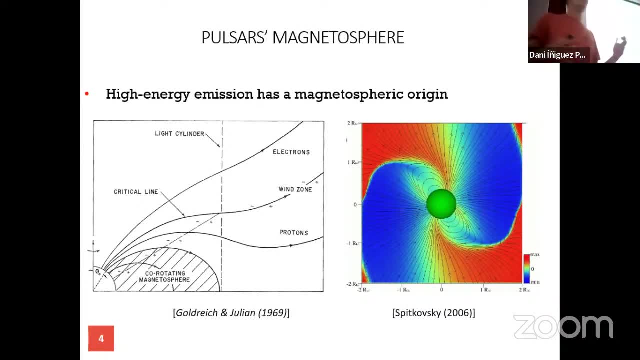 And these are what I will call high-energy effects. People ensure high-energy effects, or gaming. now, the high energy emission of pulsars is considered to be produced in the magnetosphere of a pulsar. the magnetosphere is the region embedded in the neutron star where a dynamically 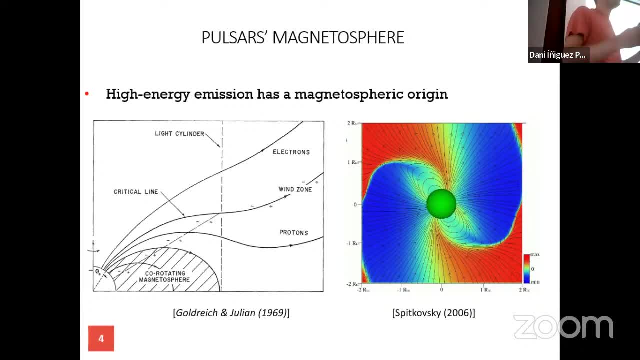 relevant magnetic field develops. this magnetic field is considered generally to be a magnetic dipole, but in reality is more likely a multiple. but this, the polar approximation, has turned out to work quite well in this region. this region is filled with such particles, which form a magnetized. 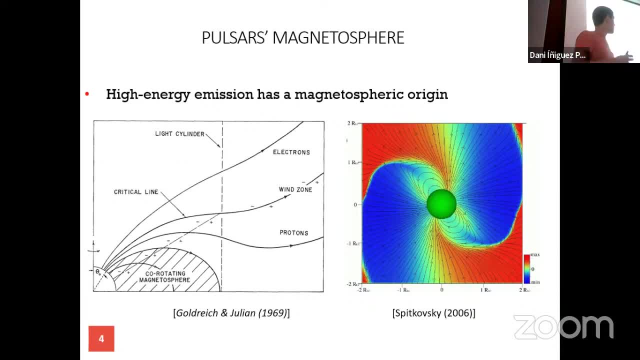 plasma, and this magnetized plasma correlates with the neutron star and up to a point at which the correlation with speed equals the speed of light. this one is the light cylinder and at this light cylinder the magnetic field lines open up, get twisted and probably undergo magnetic interaction. 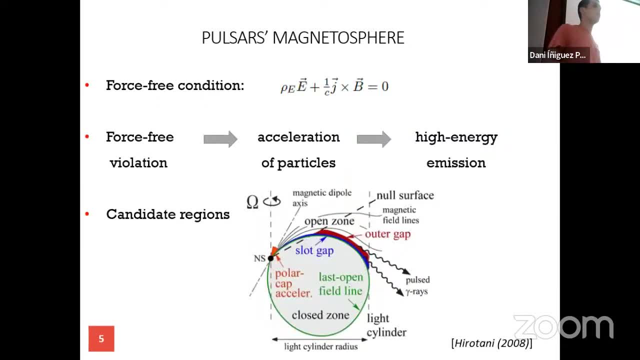 the magnetosphere is generally seen to be under the so-called post recondition, in which the Lorentz factor acting on the charged particles matches and these charged particles are thus not accelerated and slide along the magnetic field and slide along the magnetic field lines and co-locate with the stars. 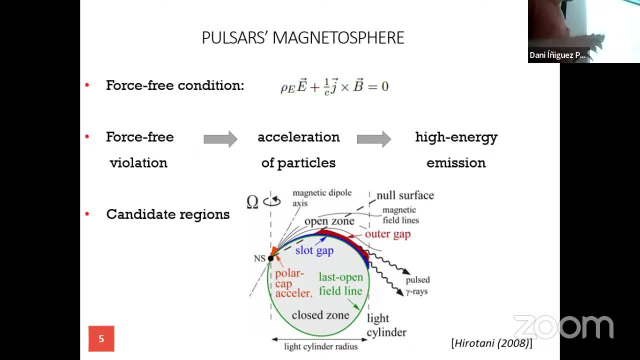 however, in some peculiar reasons of the magnetosphere, this post-leak condition is expected to be broken. when did, and probably by externalities in the plasma density? when these are fused, an electric power, electromagnetic field develops in these regions and the particles entering these regions can be accelerated. This acceleration of particles 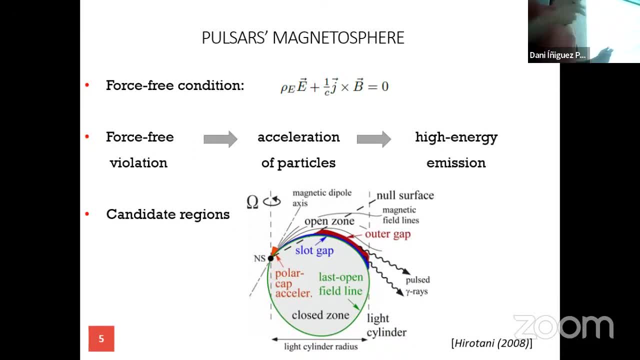 is indeed required for the dis-hygienic emission to be obtained. So in these regions where the dis-hygienic emission is violated, particles are accelerated and thus the dis-hygienic emission is reduced. Now one of the great unknowns of these negative sphere studies is: where are these? 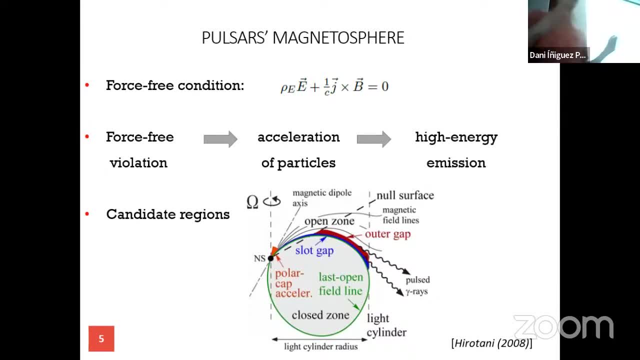 regions located. They cannot be located at any place in the magnetosphere, but instead some conditions pass 3-4-3 and thus these letters with very few candidates. Historically, the main three candidates have been the out-of-the-ramp model, which consider that the acceleration region 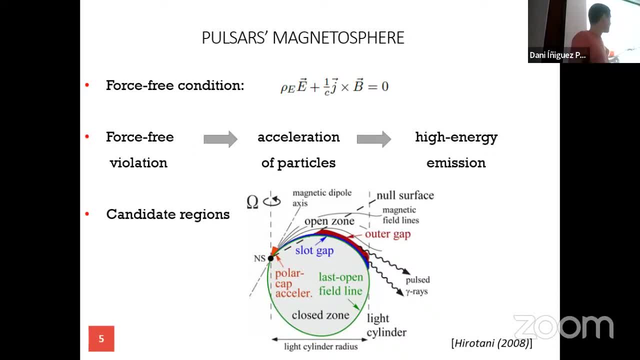 is located between the last open field line and the first open field line and has an extent of about 1 in the right cylinder. Another model proposed is the polar cap model, in which this acceleration will be located in the separatrix. Finally, 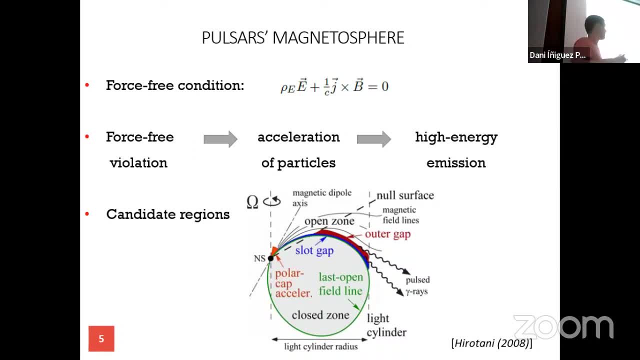 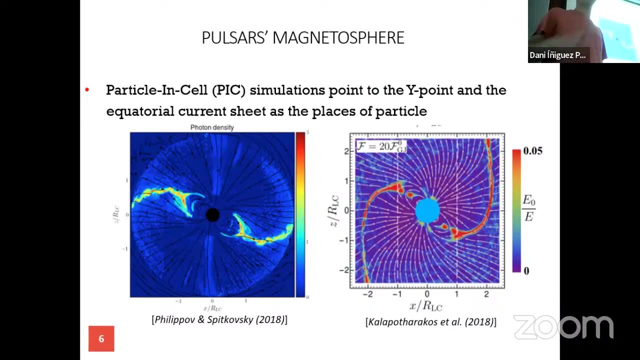 the polar cap model, in which the particles will be accelerated in the magnetic pole of the star. In the last few years, another candidate has gained force, thanks to the development of the so-called particle-in-cell simulation. These simulations simulate the dis-magnetized plasma. 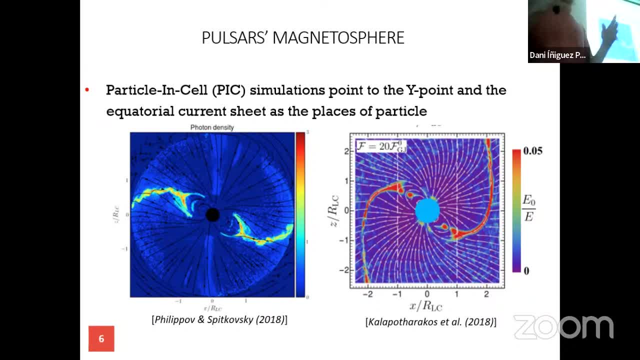 as an in-cell velocity at the top of the planet. The particle is then set up as a slit, as is done in magnetohydrodynamic simulations, which are the most commonly used magnetoscopic simulations. These particles are simulated together with the electromagnetic field in order to create such 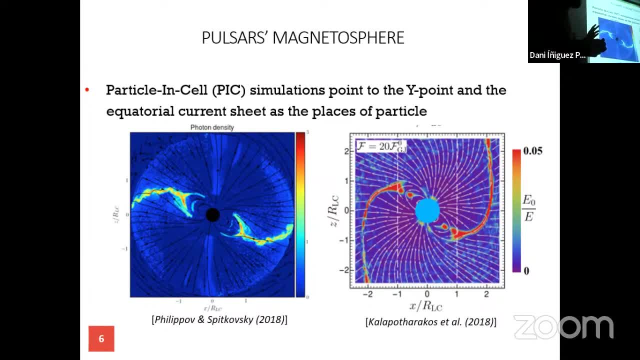 consistent magnetic spheres. These simulations done across the world by different groups all seem to point to the same places of particle acceleration, namely the white point and the equatorial part. The white point is this point here. This is where the open magnetic field lines. 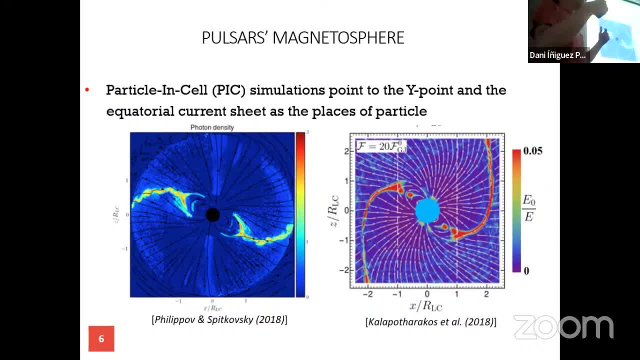 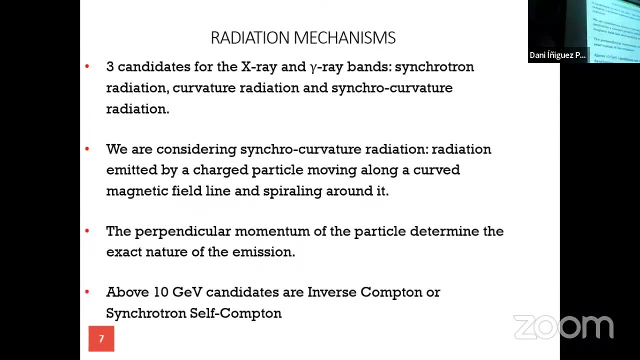 connect and undergo magnetic recognition. This magnetic recognition can accelerate particles, So in these places, this white point and the equatorial part can be accelerated and thus high-energy emission can be produced. Another relevant aspect about this high-energy emission is which is the radiation mechanism. This is the radiation mechanism, which is the radiation. 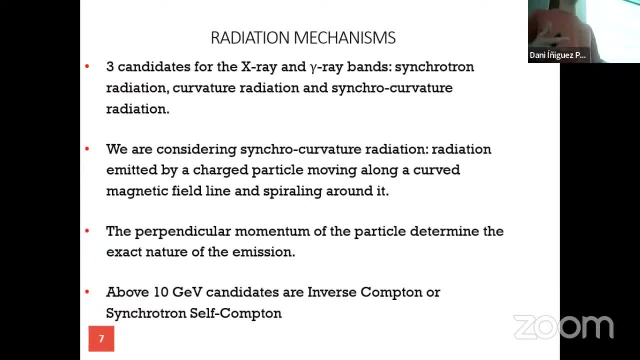 projection mechanism in action in these vision, Which is the mechanism producing this radiation? For the energy band between one Qv and the tens of Gd, x and gamma rays, the three main candidates are cyclotron radiation, curvature radiation or synchrotor radiation. This last one is the one in which we focus. 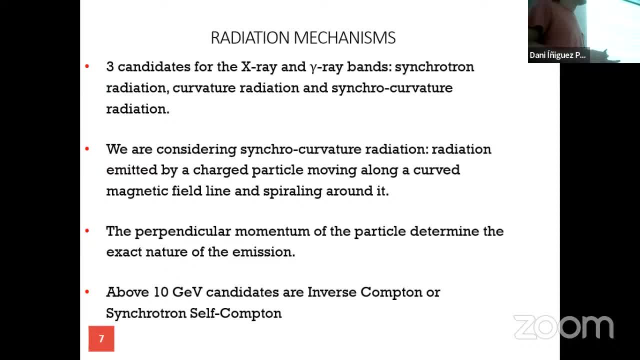 that we consider in action. It's emitted by the charged particle moving in a magnetic field line, in the curve magnetic field line, and spiraling around. The exact nature of this, of the emission, is determined by the perpendicular momentum of the particle. So the movement. 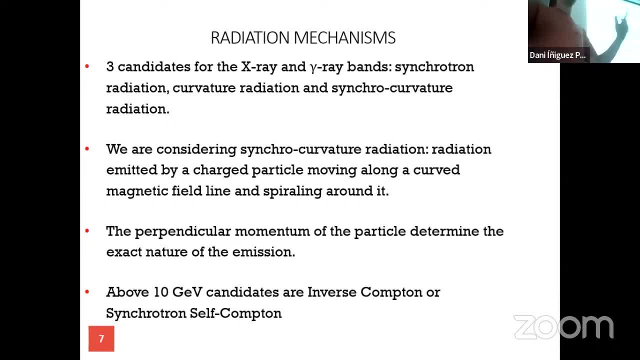 so if the perpendicular momentum is huge, the sincrotron losses will be relevant and the emission will be eliminated by sincrotron variation. On the other hand, if the perpendicular momentum has been totally lost and the particle slides parallel to the magnetic field, 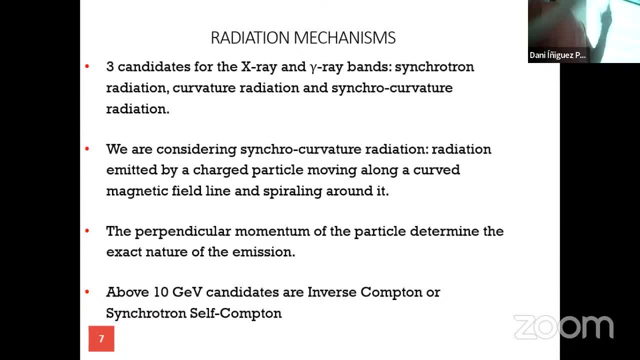 the variation will be eliminated by curvature. In the situation in between in which there is a perpendicular momentum, that is not very relevant. the emission will be purely sincrotron. sincrotron And for higher energies, about 10 dBs and up to 50 dBs. 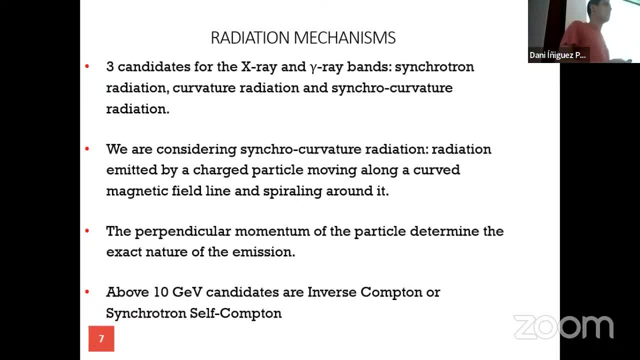 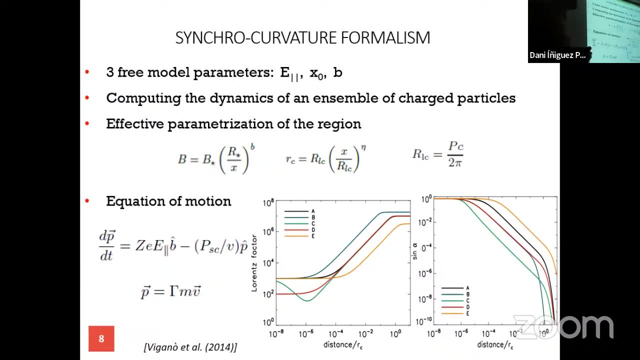 the main candidates proposed are the intercontinental scattering or the sincrotron set from there. Now they have said what we are considering is this: the sincrotron-vascular variation. So we base our model on this kind of variation. Our model relies basically on three effective parameters. 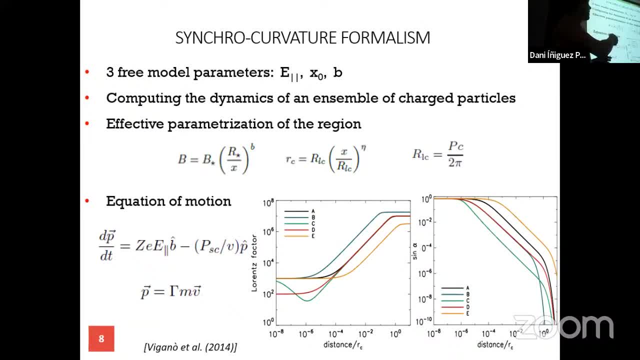 the parallel vector field in the region and an effective length scale of the region-to-region and the local strength of the magnetic field in the region. With this effective approach, we are able to reduce the complexity of the problem for three parameters, which make our model much more easy to handle. 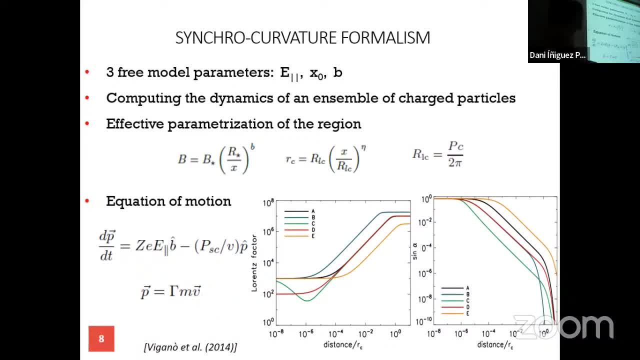 And that's what we're actually going to do. What we do, first of all, is to compute self-consistently the dynamics of an ensemble of such particles moving along magnetic field lengths in these acceleration regions, And we consider that all the particles travel. 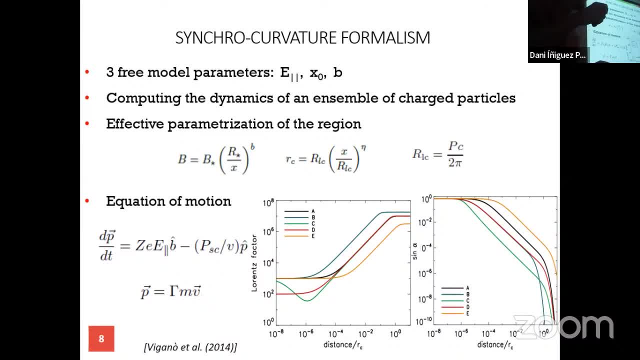 back in the backward direction, so as in the neutron star, And all are born with the same properties, namely an initial value of the Lorentz factor of 1,000 and an initial value of the Lorentz of the pitch angle of 45 degrees. 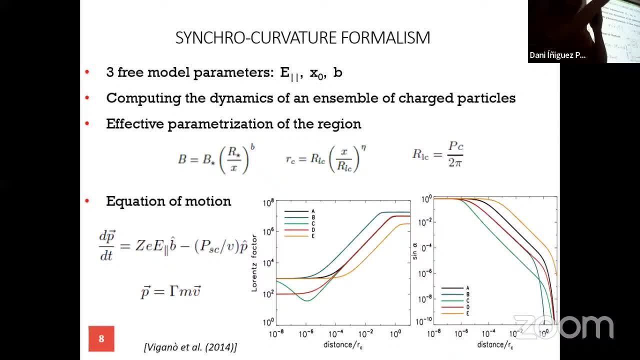 The pitch angle is the angle between the direction of motion of the particle and the direction of the magnetic field. Now we characterize our acceleration region by effectively parameterizing two relevant quantities: the curvature value of the magnetic lines in the region and the local strength of the magnetic field. 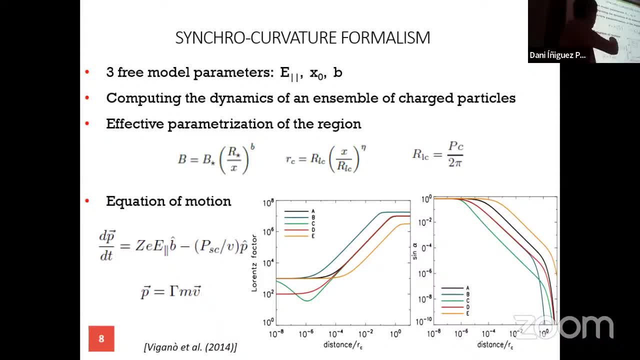 along this region. We do so with this two-order parameterization, in which this parameter V is the so-called magnetic gradient and is one of our three parameters. Once this parameterization and the initial conditions are established, we let to numerically evolve the ensemble of particles along the region. 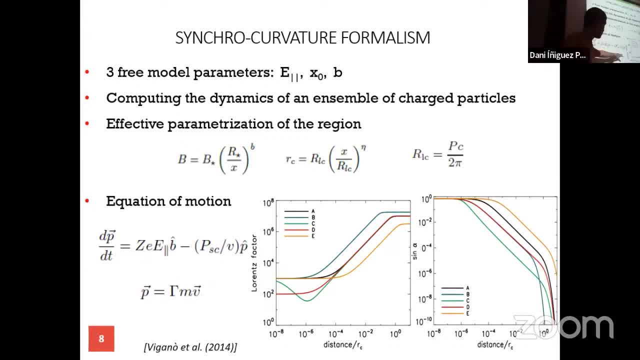 with the evolution ruled by this equation of motion, in which this term is the radiation reaction force That accounts for the cyclotropic losses that suffer this particle when they are accelerated by this electric field. This parameter, that I will call a parallel, is another of the three parameters of the integral. 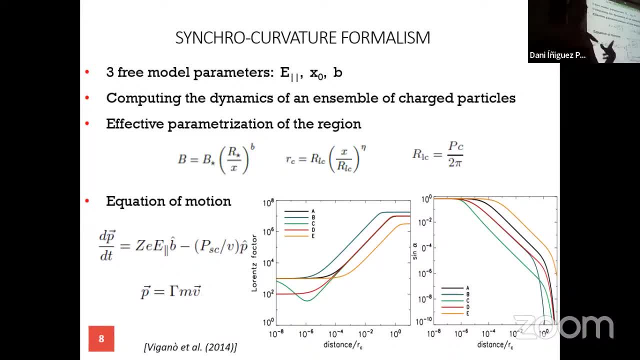 Then in this way, with this equation of motion, we get the evolution of some part, evolution along the region of some element-magnetic quantities, For instance the Lorentz factor of the particle. you can see here how, the distance, the increase. 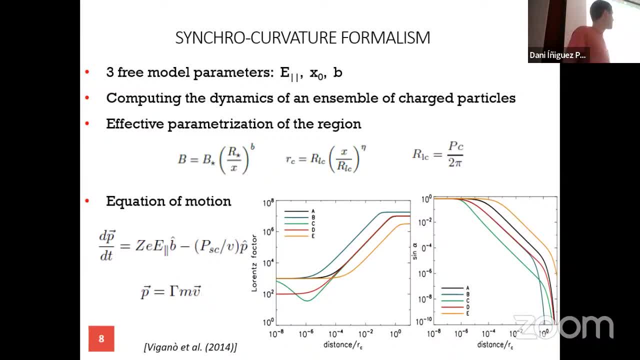 the particles are being accelerated and that's the length of the increases and also the pinch angle which lets you go over the increases in distance, meaning that the perpendicular momentum of the particles has been lost, but is being lost due to the loss of perpendicular momentum due to cyclotronic losses. 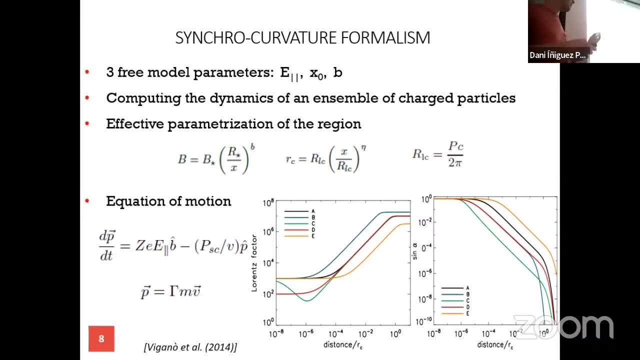 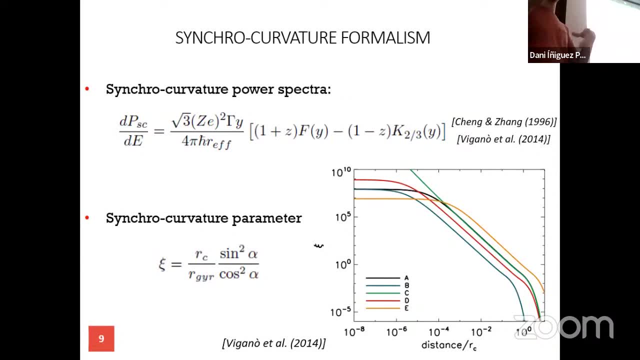 Now having the evolution of this kinetic quantity allows to compute the spectra of a single particle at its position of the trajectory. This is done by use of the simple curvature formalism which was introduced in 1896 and formulated here at the time of the 1315.. 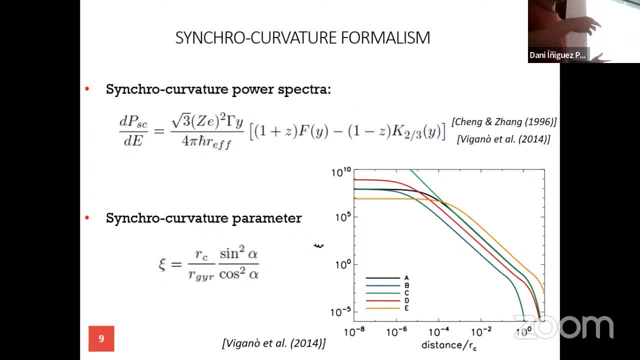 And this is the expression for the simple curvature of the power spectra for a single particle. And this formulation right here it can use a key parameter, the so-called simple curvature parameter, which indicates the nature of the radiation, that is, for the simple of curvature. 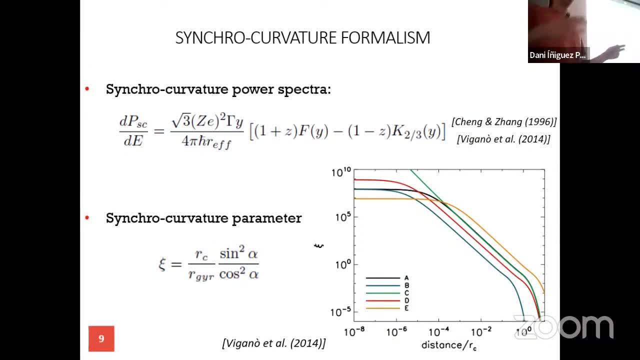 it's only the emission, And for large values of these parameters, the of this parameter, simple coordinates, and for small values of this parameter, the curvature is the dominant radiation. You can see here the evolution of this parameter along the region, So at the beginning of the region. 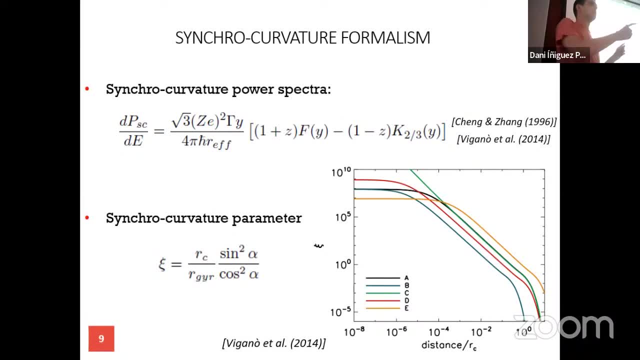 then this parameter is large. So the net force of these trajectories, then the dominant radiation, is simple, While the other parts of the trajectory the dominant radiation is, And in between you have this transition region in which the emission is purely simple, simple color. 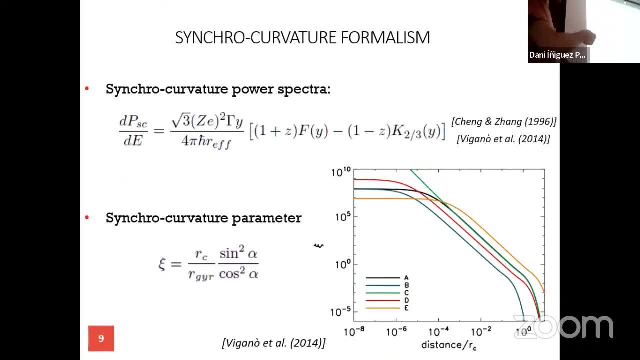 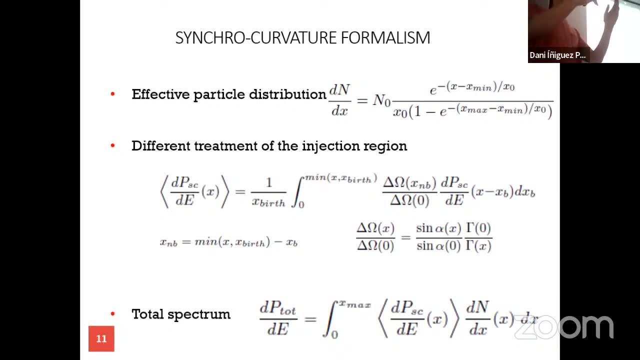 And these are the magnitude of this and the spectra, And in order to account for the diversity of magnetic field lines and of trajectories present in the region. what we are doing is to giving a way to reach to the contributions of each of the points. 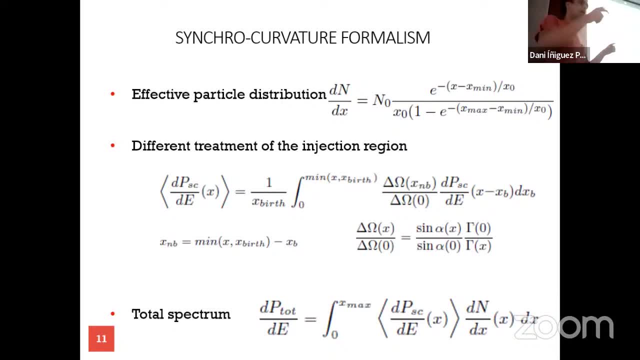 in the trajectory. In this way, what we are doing is this practical distribution, And in this way we are reducing the complexity of the real scenarios. So we are using some physical ingredients that we are not considering And we are able to contain all this complexity. 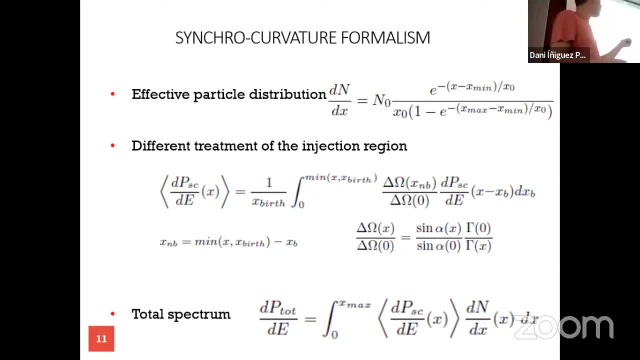 in one effective particle distribution, And this one parameter is zero. This contains all this complexity. This parameter, in the concept of this optical distribution, indicates the greater of the uniformity of this distribution. So for small values of this parameter, more weight is given to the inner force of the trajectory. 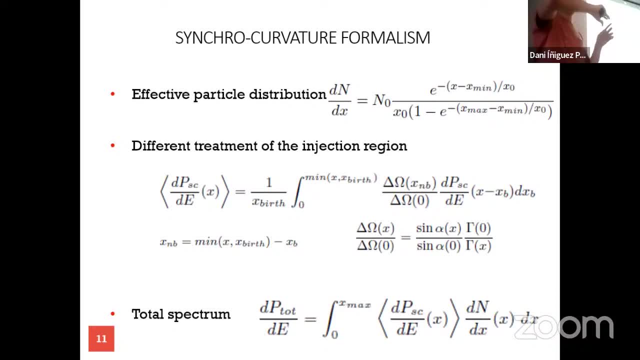 while a larger value of this parameter indicates that the distribution is more uniform along the acceleration region. Now, one physical ingredient that has been newly introduced in the last year is a different treatment of the injection filter. What was done so far was to consider that. 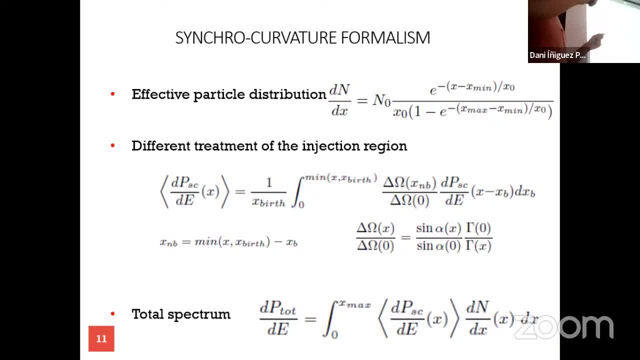 up to an extent of 10 to the minus four light cylinders, all the contributions from all the at each position, the contribution, the spectral contribution, was eliminated by the properties of the particles being injected at each one of these positions. But what we do now is to consider properly. 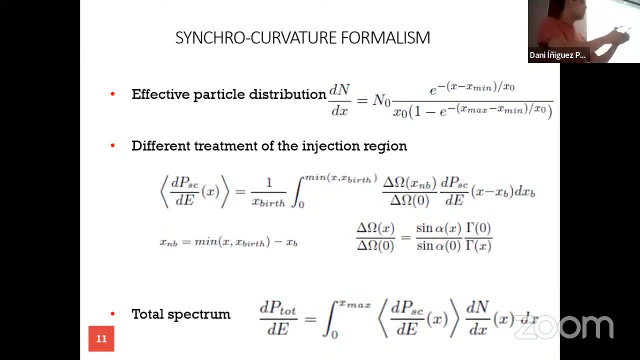 the trajectories of all the particles, so that at each position of this so-called injection region there is not only the contribution of the particles being injected there, but also the contributions from the particles that are injected at inner positions in the trajectory. So there is this at each position. 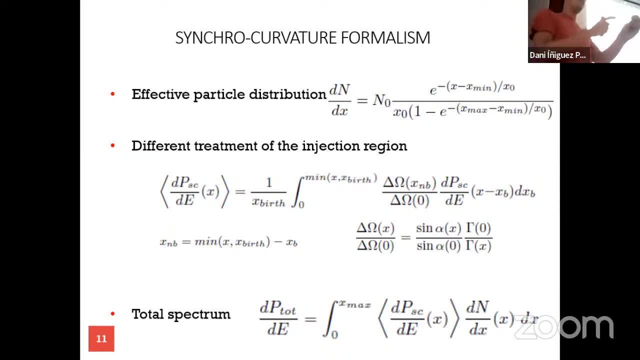 there is a contribution from the particles being injected there and the contribution from the particles being injected at the inner positions. To account for this effect, we introduce another wave and we convolve our simple particle spectra with this wave and after that we convolve this spectra. 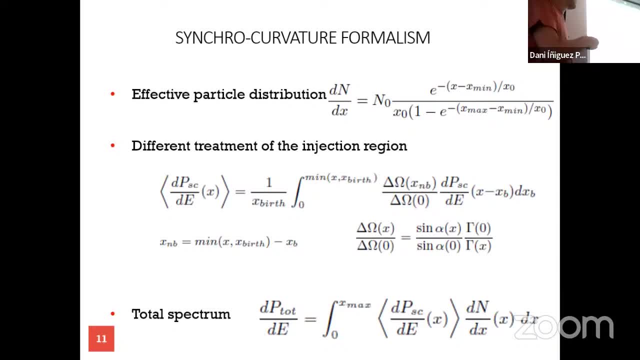 with the spectral distribution that I have mentioned. now, I always forgot to mention about this in general: the normalization of the distribution that is simply as scaling factors And some analytical. So when we conv dissociation of this wave, you obtain the total expected. 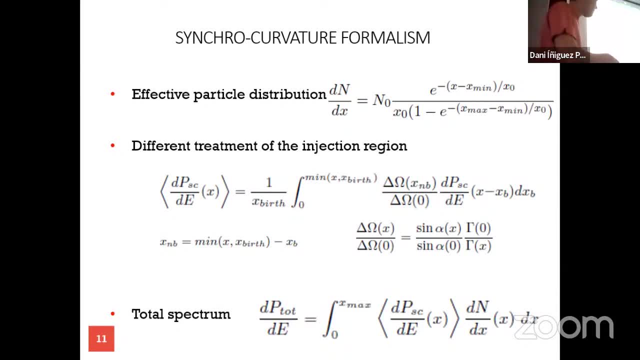 inter-virus countries. So that is the fact, is this one and this spectrum. so that means zero. with another parameter, that means 0.. of this spectrum is ultimately defined by only three parameters: the e-parallel 0 and the magnetic gradient V, and this normalization. 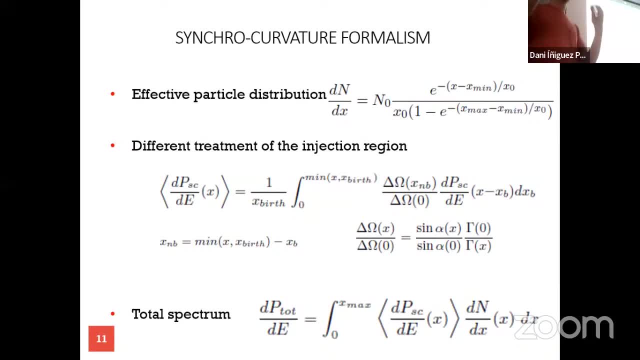 So that we are able to describe the spectral energy distribution of a particle of a producer soil, with only three parameters and normalization. Now, in order to compare our spectrum with the real spectrum, so to assess how similar are the spectra produced by our model to the observational spectral energy distribution of pulsars. 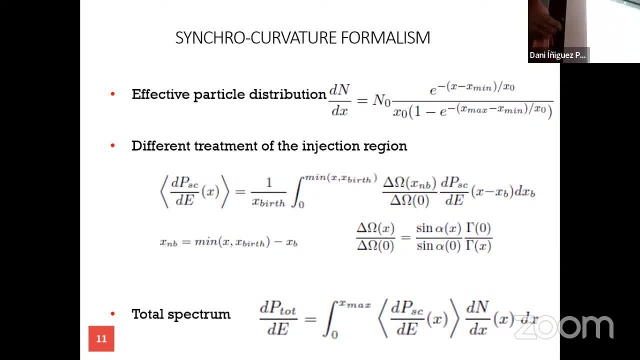 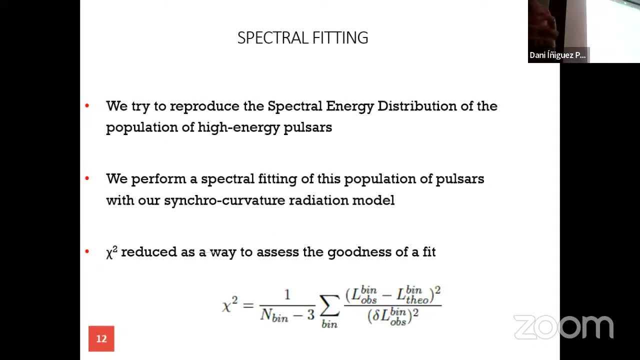 we have to confront our model with real data of high-energy pulsars. We do so by fitting the population of high-energy pulsars with our model. We do a systematic analysis. This is the fitting of all the population, thanks to the effective approach that allows to constrain the model parameters. for all the parameters. 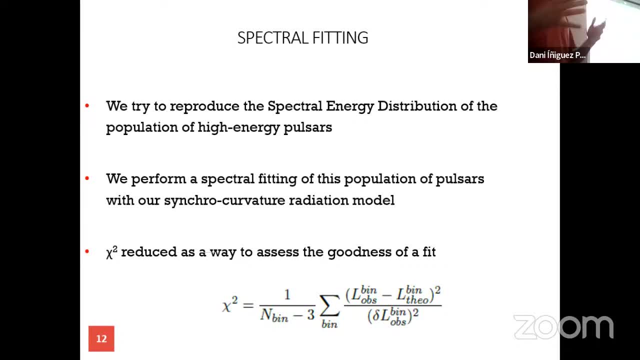 In order to assess how good a fit is, what we do is to consider the statistical chi-square radius. This is the spectrational luminosity and this is the error of the spectrational luminosity. The first one is the theoretical luminosity produced by our model. 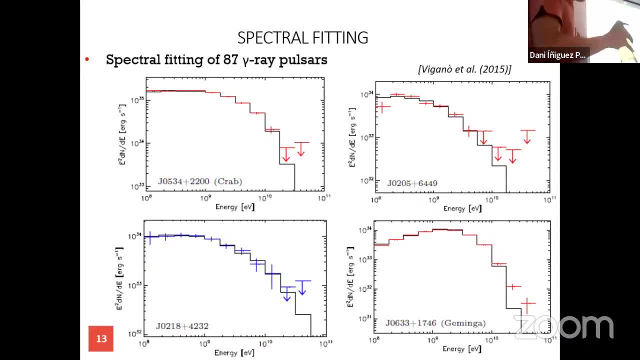 The first one of these spectral fittings was done in 2015,, in which a sample of 87 gamma-ray pulsars fit with data produced by our model, And the model successfully resembles this spectra quite good. These are some examples of the spectra of the fittings back then. 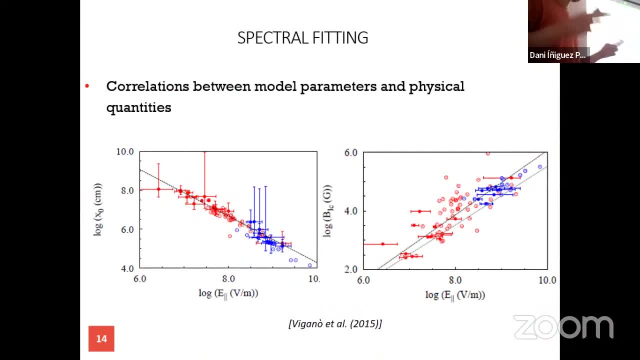 Also in this paper there was a study of the correlations between the model parameters and some typical number between the pulsars. We get these two correlations, an anti-correlation between the two model parameters E0 and E5. And also this correlation between the parallelepiped field and the strength of the magnetic field. 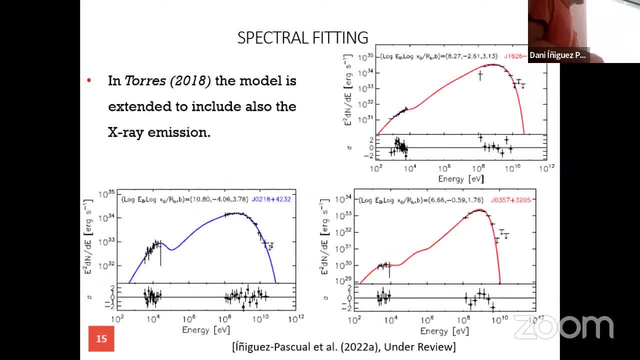 After that, in 2018, the model was extended. We used also the X-ray variation, That is, with our theoretical spectrum we could reproduce both the X-ray and the gamma-ray bands spanning 8 orders of magnitude. Then again in 2019, was done a spectral fitting of the pulsars. 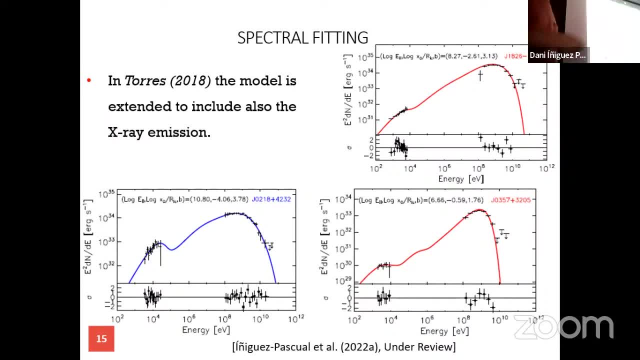 processing both the gamma-ray and the X-ray data, And these spectral fittings have been repeated now this year, with the same results and a more concise treatment, And in this fitting the majority of the pulsars were reproduced by our model. These are some examples. 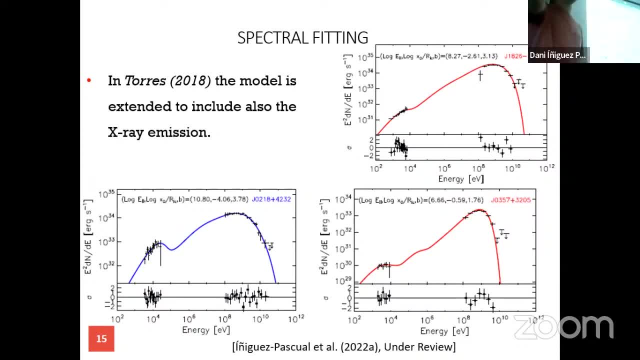 Both bands are reproduced quite well by our spectra, And this is remarkable because a few of the radiative models that exist are able to reproduce both bands at the same time and with a single radiation mechanism. However, not all the pulsars were well fitted. 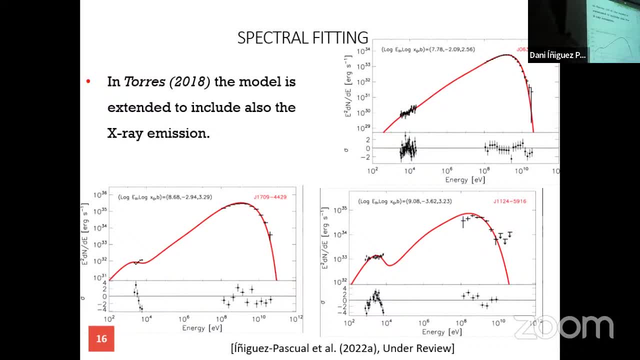 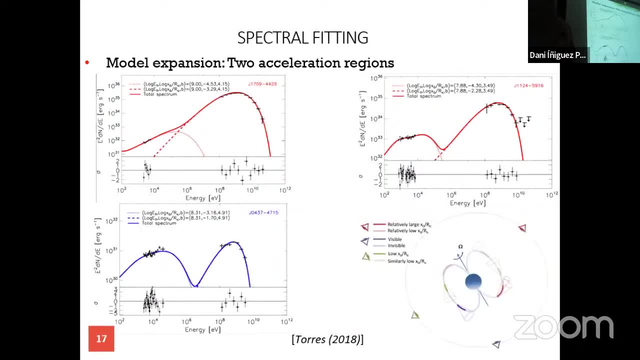 In some of them, the model was not able to reproduce exactly the data Here, And for these cases we proposed an extension of the model. Instead of considering one acceleration region, two acceleration regions were considered, So that the radiation we detect from Earth is the sum contribution of the radiation emitted from both accelerators. 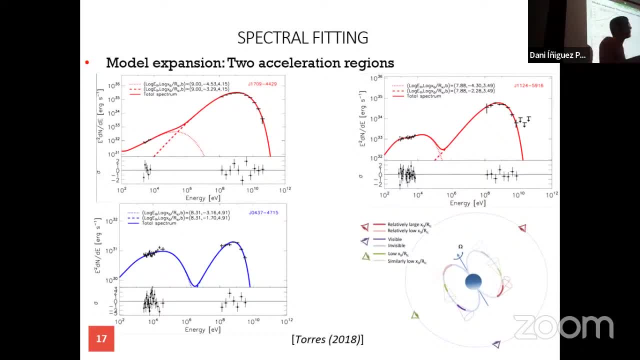 This is a schematic representation of how this situation could be In our spectral fitting. we are not doing any strong assumptions about this, So we are not getting information about the geometry of the radiation. This is just an schematic idea And with this model, with the expansion of the model, the pulsars were not well reproduced by the model with three parameters. 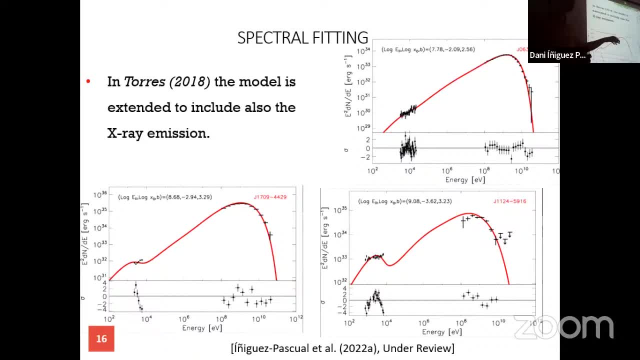 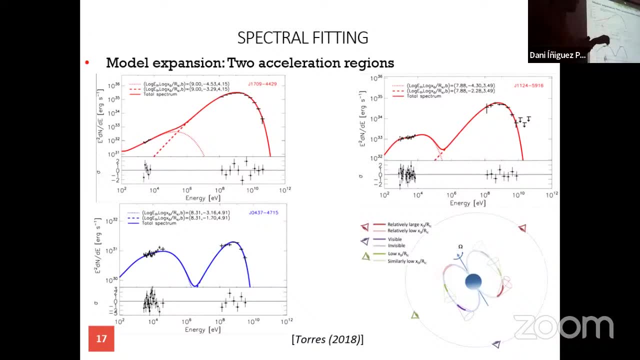 We call this model with three parameters a minimal model. So the pulsars were not well reproduced by the minimal model. Now we use the expansion of the model, well reproduced, As can be seen clearly from some of the radiators. Then in the last few months another expansion of the model was proposed. 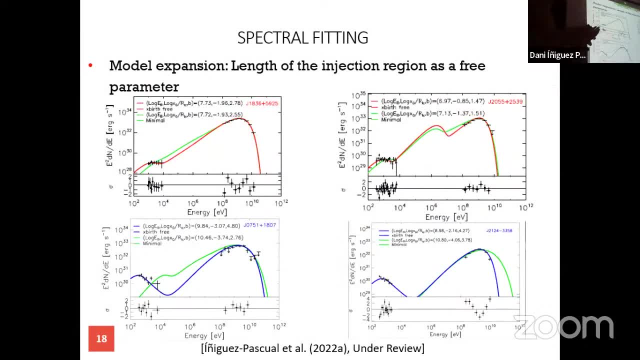 We asked ourselves if letting the length of the injection region that I have mentioned before as a three parameter in the synoptics could be used to to explain the pulsars that were not fitted with the minimal model. So we did so And for some of the pulsars that were not well fitted with the minimal model were now fitted. 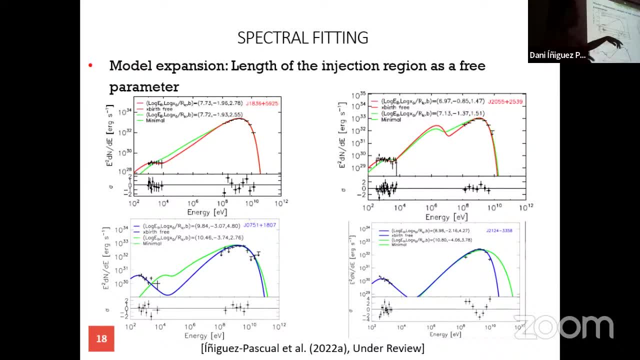 We have. the green lines indicate the type of fusion by the minimal model, And the red and blue are the models in which the injection region is left free. Some of the pulsars were well fitted, Not all of them, So that if we were to choose an expansion of the model, we would rather choose the one with two acceleration fusions. 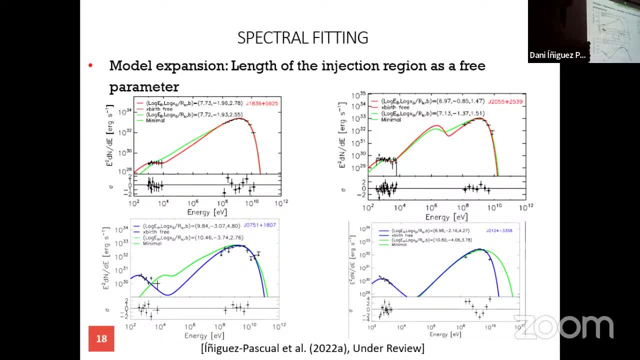 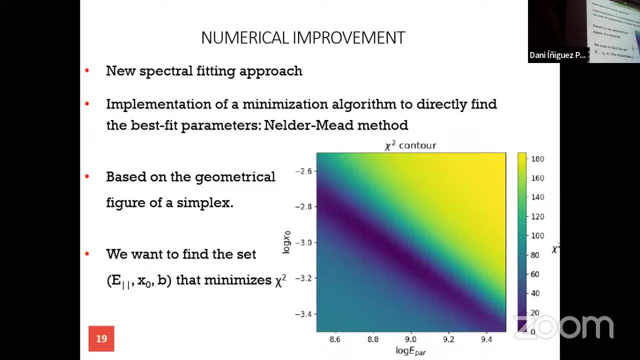 instead of the one in which the length of the region is the same. Now let's move to a more numerical aspect of our project. About a year ago, we thought on including the numerical approach, the numerical procedure that we were, that was being used. 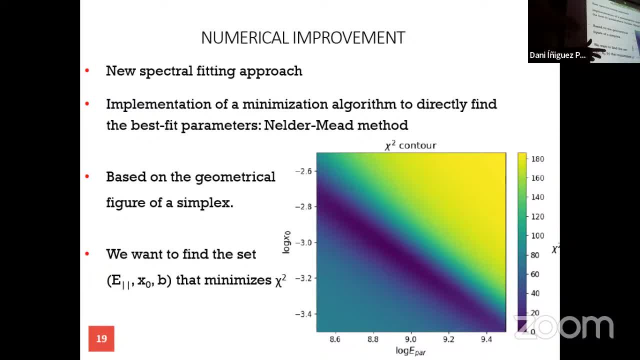 And we implemented an administration algorithm in order to directly find the rest of the parameters, of the, the parameters given in our field. The algorithm we introduced was the Nelder method, which is based on the geometrical figure of a simplex: A simplex in two dimensions with a triangle, and three dimensions with a vertical. 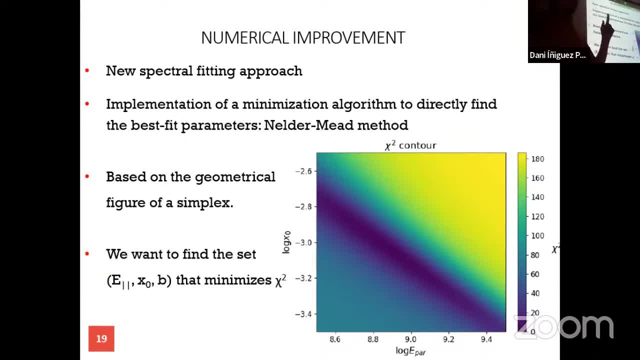 So this simplex is placed in the space of parameters which in our case are parallel- b0 and b- And at each of these vertexes can be evaluated the function to minimize. In our case, the function we want to minimize is the chi-square radius. 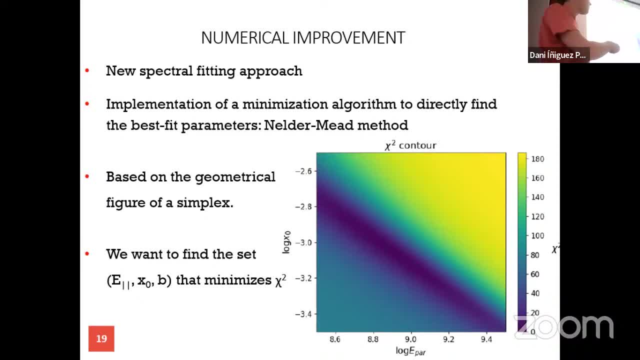 which you can see. here is an example of how it works in three dimensions. So what we want to do is to find the set of model parameters that minimizes the chi-square, In order to find this minimum. this simplex is led to evolve. 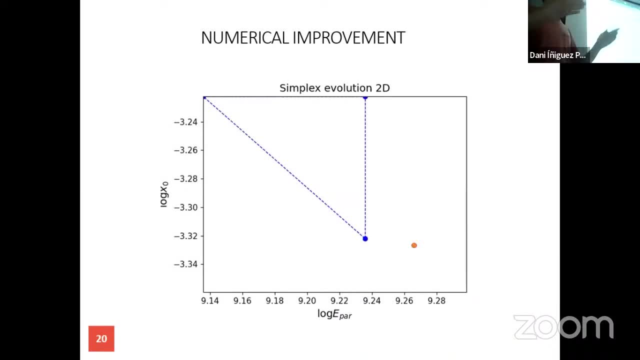 being iteratively modified with a series of transformations, and is directed to the space of parameters and to the region of the minimum. Here you can see how this evolution goes. The simplex is modified, it reaches the region of the minimum and reaches this region. it spins, it swings. 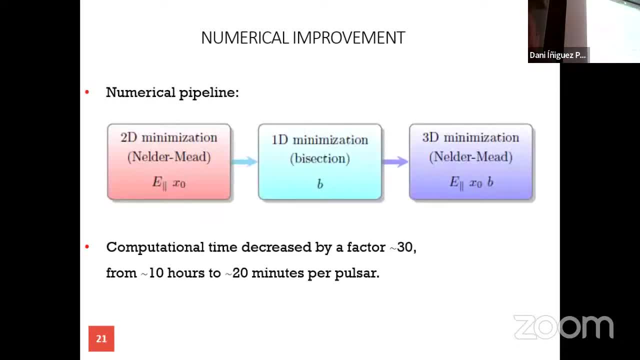 and finds the minimum. Now we implemented an American pipeline consisting of three different steps. The first one was a two-dimensional Melder myth in which f- parallel and x0 were led free and b was fixed to a crucial value of 3.. 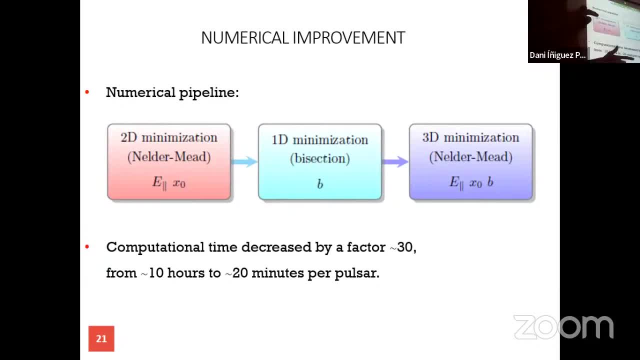 After that, a one-dimensional section in which b was led free and f parallel and x0 were fixed to the basic value from here. And finally, a 3D Melder myth minimization, where all the three parameters were led free. 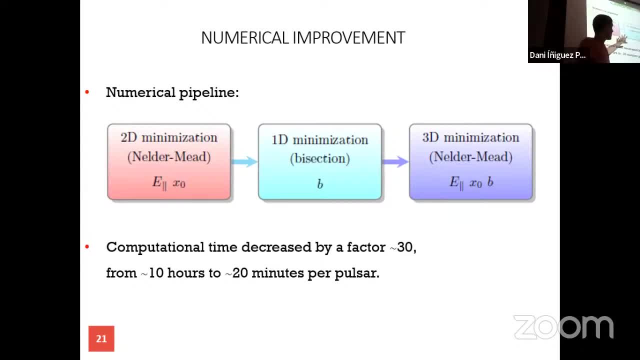 We decided for this configuration because with this two-phase step, we are already close to the region of the minimum and with this last step we are continuing the result and ensuring that the results found, the minimum found, is good. This reconfiguration was the better fit. 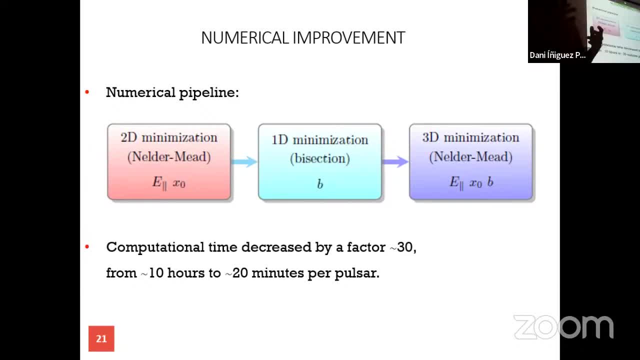 between computational performance and security of the minimum we have found, which is applicable Now with this new approach. the computational time decrease achieved was of a factor of 30, depending on the exposure. This translated to a feeding time of now 20 minutes. 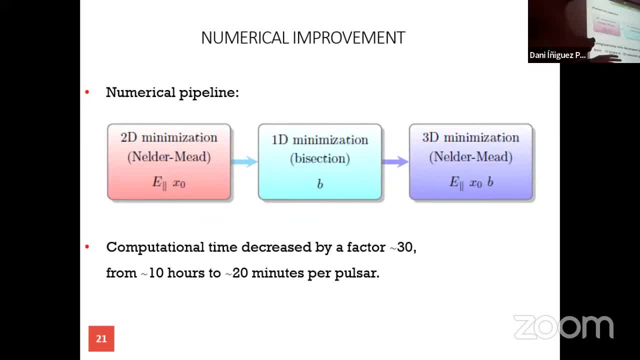 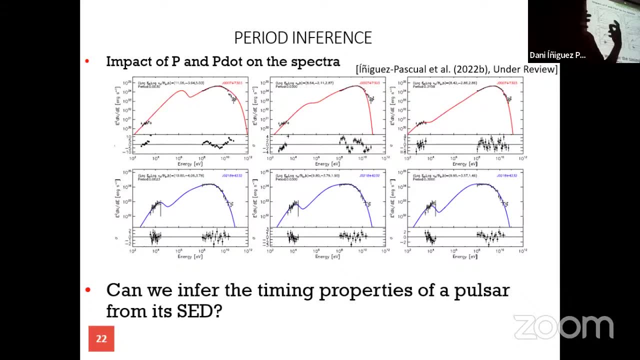 while with the previous approach it was 10 hours. This numerical approach allowed us to get engaged in more computationally demanding studies, For instance, one related to the timing properties of the filters. We focused on these timing properties, namely the period and the period derivative. 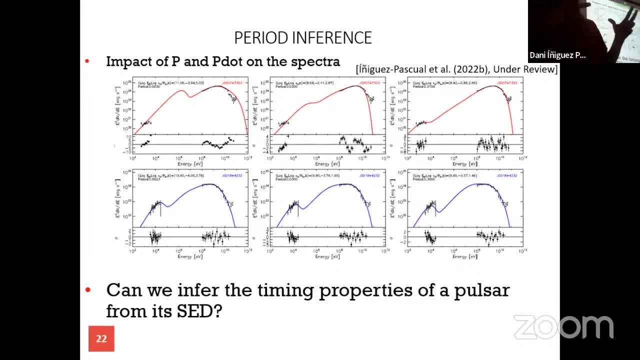 and we studied how these timing properties affect the spectral energy distribution of a filter. In order to do so, we took a pulsar, which is the phase of the second phase, which is the phase of the second phase plus the phase of the third phase. 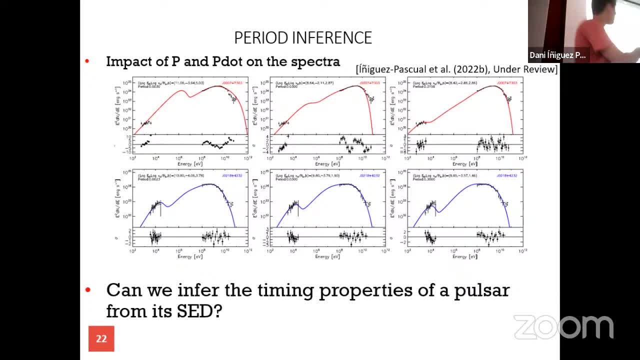 and we changed its period. So we considered the real period, which is 560 milliseconds, then 50 milliseconds and 50 milliseconds. For each one of these different periods, we perform a spectral activity and these are the results we obtained. 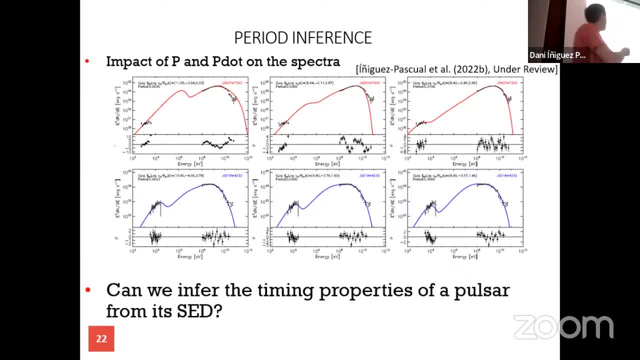 For the real period, of course, the activity was good, but for the other two periods, the best things- fun- cannot be considered as a good thing. So what does this mean? The same is observed for the second project, and not that clear. 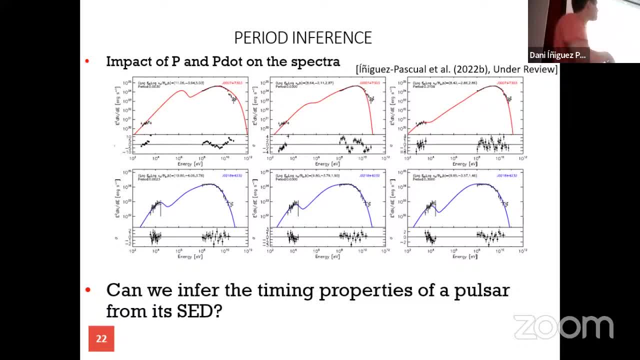 as in the previous seven, but okay. So what does it mean? It means that if we do the exercise of not considering the period, the period of a pulsar- and we do the spectral activity for three different values of the period, 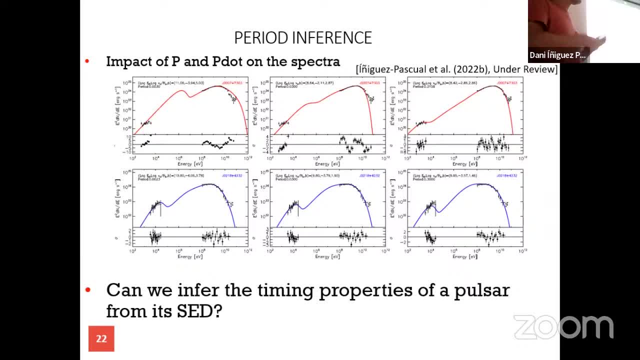 we were able to. we are able to say which is this real period. So if we watched these three results, we would say that the real period is this one, or at least it is close to this period, because the spectrum is quite better. 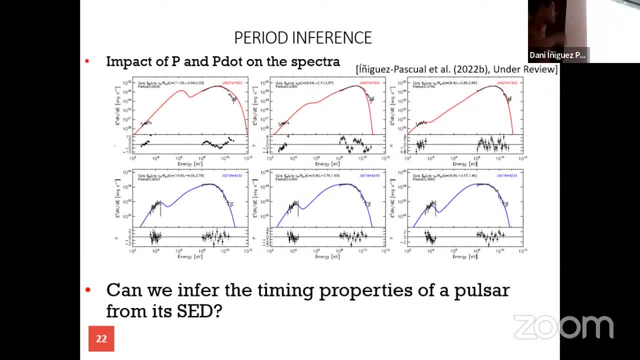 in those in this behavior. So in light of this, we asked ourselves: can we infer the timing property of a pulsar from its spectral energy distribution, That is, if we are blinding ourselves from the timing properties and just considering the spectral energy distribution? 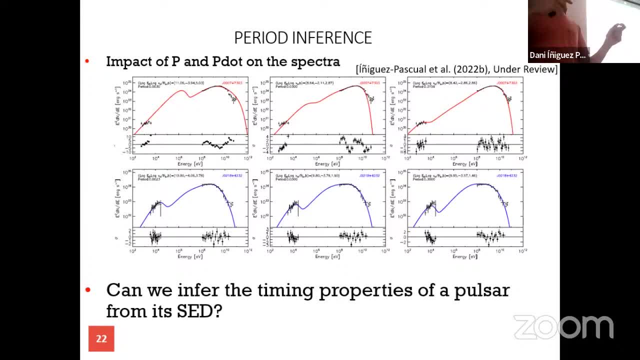 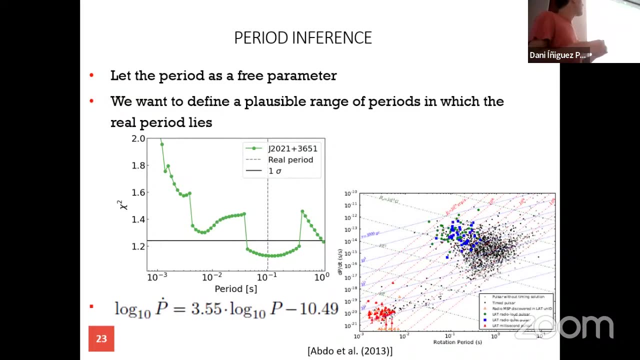 we were able, if we are able, to recover the timing properties of the pulsar. So some hints about the, about the real period of the timing property. In order to ask these questions, we modified our spectral computing tools in order to use the period as a free parameter. 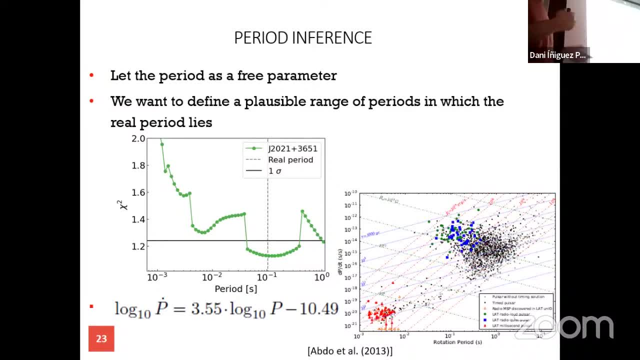 To do so, we defined it a logarithmically spaced width of periods from one millisecond to one second, because this is the typical period range of gamma-ray pulsars, And for each one of the periods we performed a spectral activity, so that we ended up with 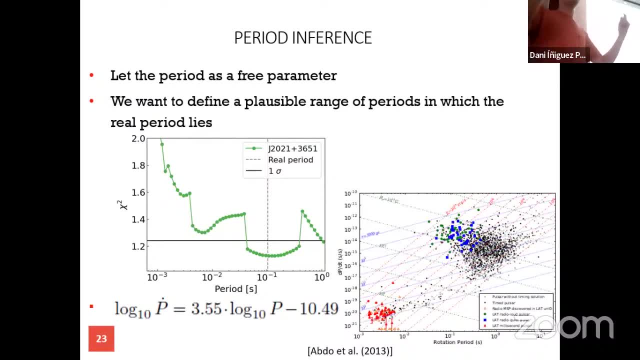 a width of period and for each period a value, a chi-square value. With this it is possible to draw a chi-square versus period plot And we, with this, we went at defining some a flexible range of periods in which the earlier period lies. 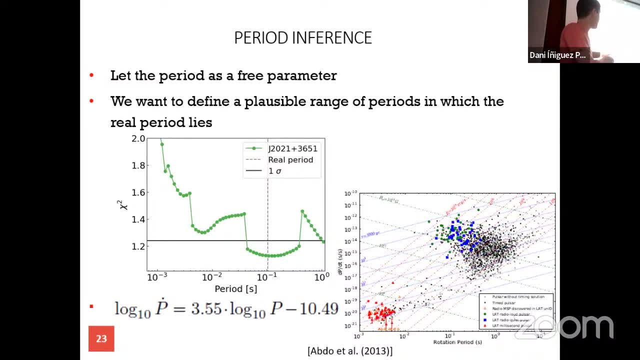 So this is our our goal: to find something like this in which, in this period, the dashed line is inside the range. The range is defined with this amyloid, which indicates at one signal distance from the the smallest chi-square. 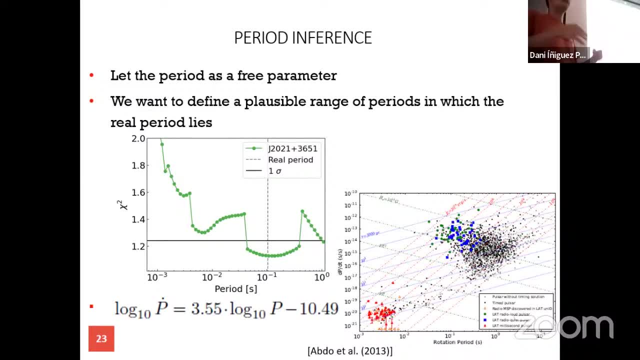 So that all the points below this this line are statistically equal in widths. So in this range of periods we will place on the period that lies below this line. So notice that if we are planning our set from the timing properties, 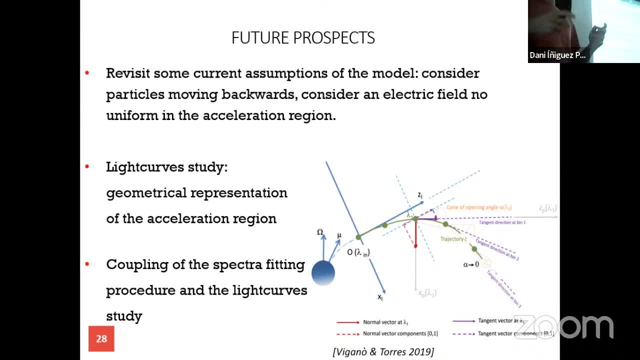 theoretical structure and some studies have been done. So our plan is to continue with these studies and the near filter and coupled the spectral shooting procedure with this light curve study in order to obtain much more information about the objects we are studying and improve our knowledge about the higher resolution of uh, the higher resolutions of photos, and that's all we. 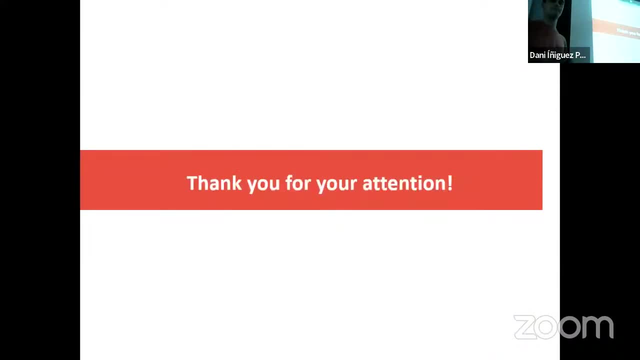 for today, okay, okay, so, um, okay, what i assume. and the question is: which is the error in the estimation of the period in this period, inference application? But we are not giving an exact value of the period, So there is not this error. What we do is only defining a range of periods. 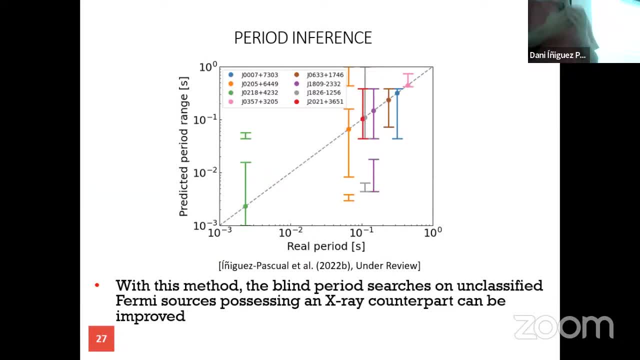 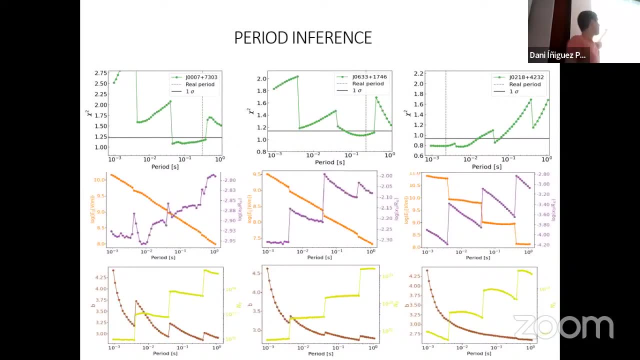 in which this period may be located. But since all these points are below the AMNI limit, we cannot statistically say that some are better than the others. So we are not doing any assumption about the exact value of the period, But instead of giving an array. 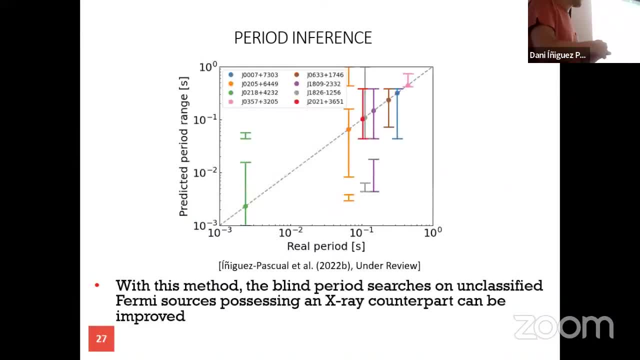 we just relate it to the expected error. So the question is, which is the real period estimated? The question is that I don't really know, because I don't know expert on this observational site, but i don't, i don't really know. i feel that that it is. 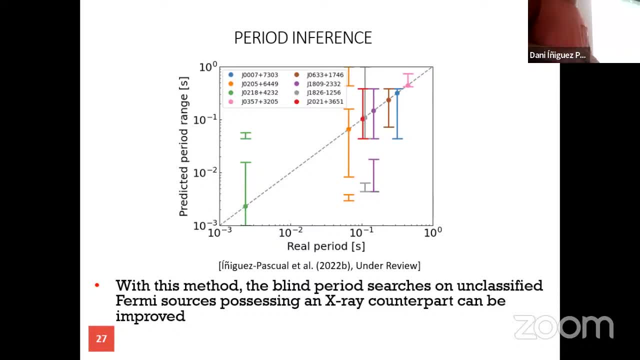 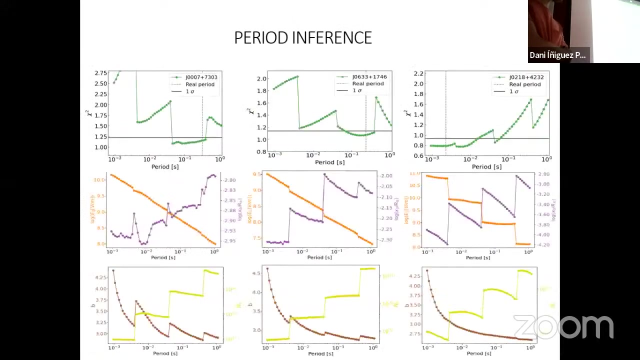 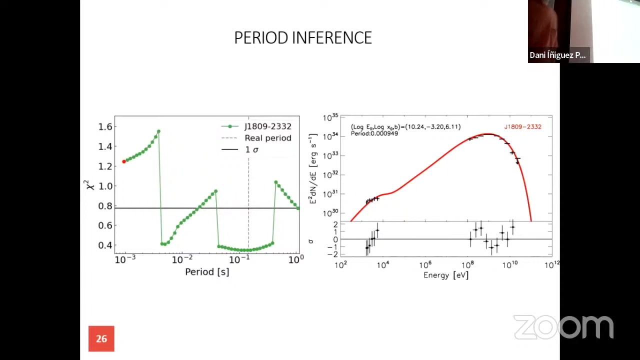 how can? i is the new time, and then they learn from this particular? yes, any other questions? uh, video. well, this is not exactly pretty similar that the the spectra changed abruptly, so this is a result of the model trying to accommodate more increasingly uncomfortable situations. so, um, In here the feed is going a little bit back, because no other combination of parameters gives a better feed. 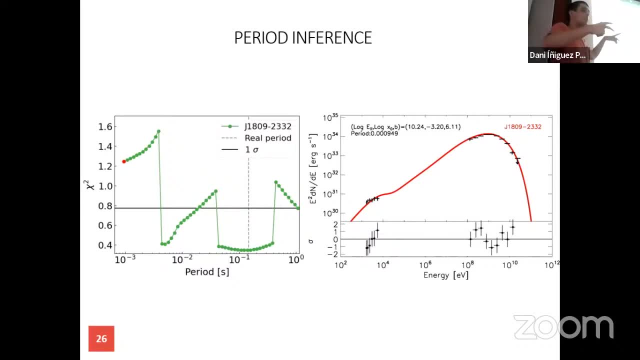 And at this point the cache-per-reduce changes and another minimum- better feed- appears, and then the algorithm points to this other minimum. And we have tested like this and we have got local minimum. so it is clear that the function changes. 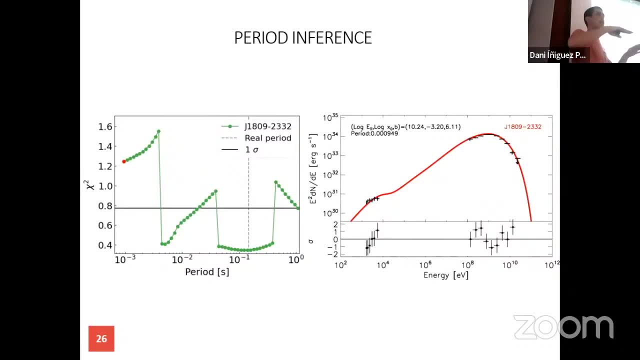 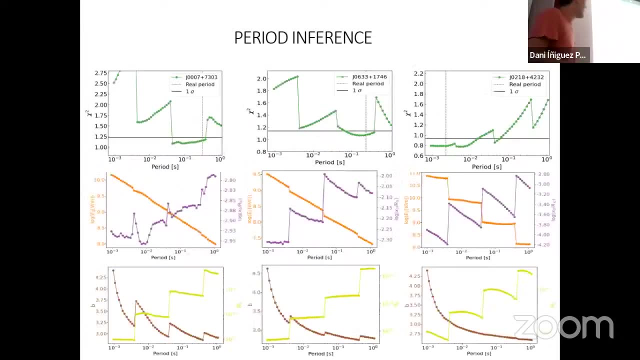 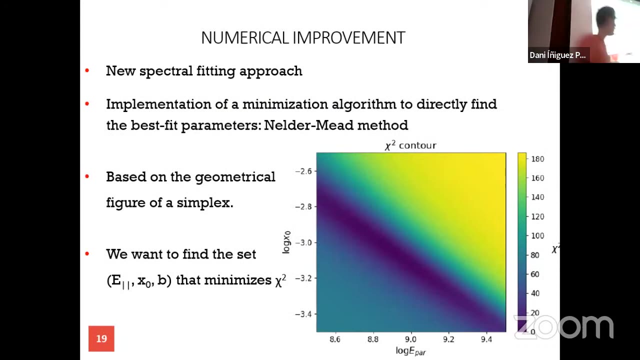 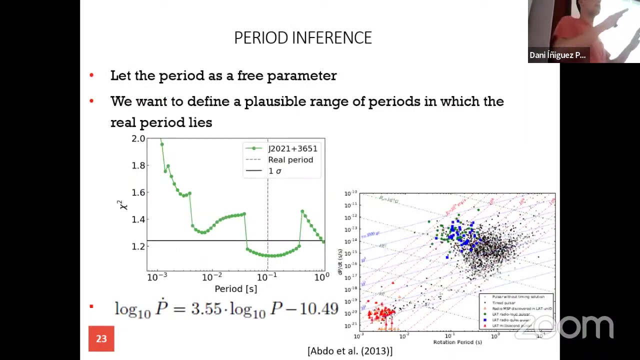 and for this period a minimum appears. that was not present in this algorithm, So with only a parallel 0 and b, the cache-per-reduce function is quite small, so it is quite valid, but when adding the period this smoothness kind of disappears in some region. 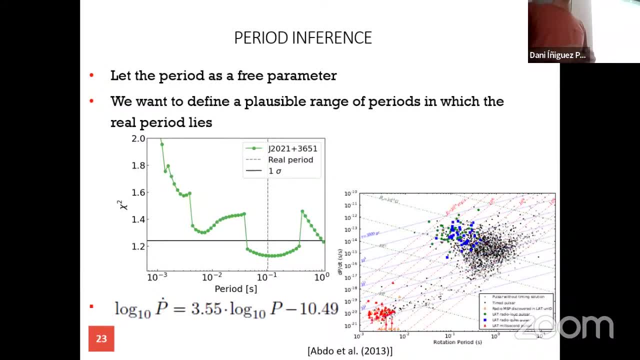 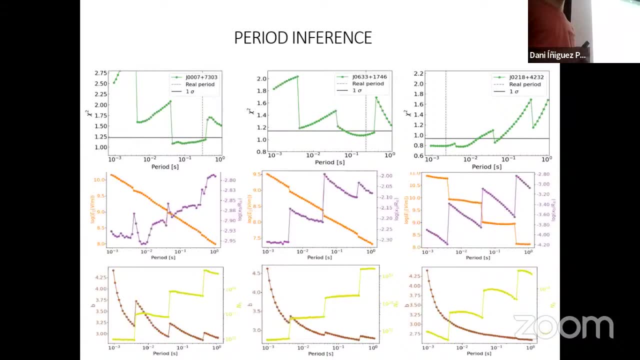 so this algorithm changes? Yes, exactly. This is a short video and it is Yes, exactly So, taking the Bessel parameters of this period, this period gives a worse feed than the Bessel And all these jumps remain. 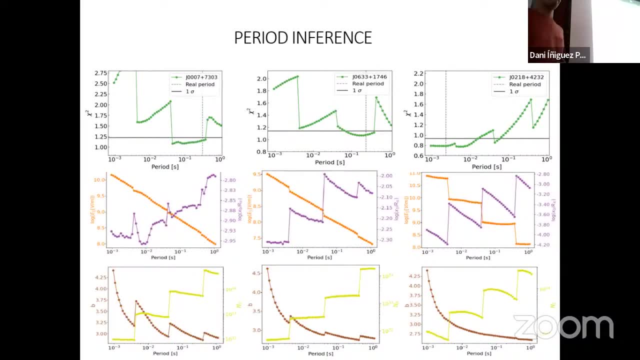 Any other questions Also from Zoom In Zoom. any questions, No questions, No questions. At present, you are just considering No, no, Yes, Yes, You are considering synchro- and synchro-curvature radiation. 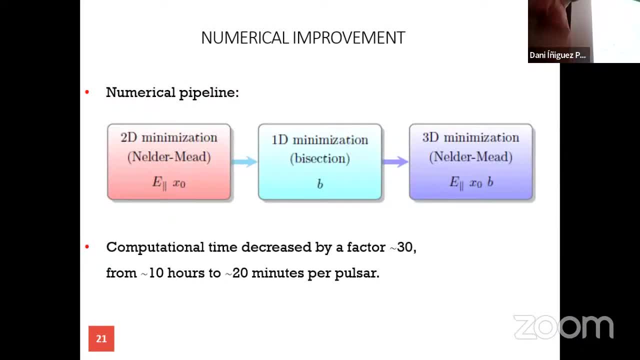 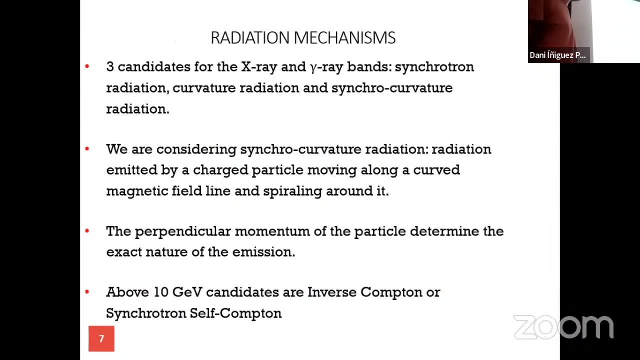 but this is one of the few perspectives for the NoSolNeur data, I mean this inverse quantum and the axial synchro-curvature quantum, In order to explain also these, all these fails that appear in the Например technique. 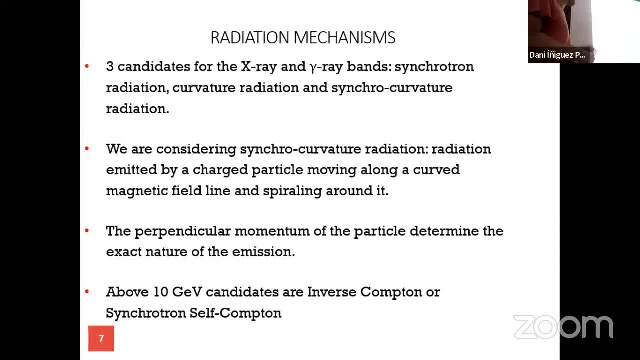 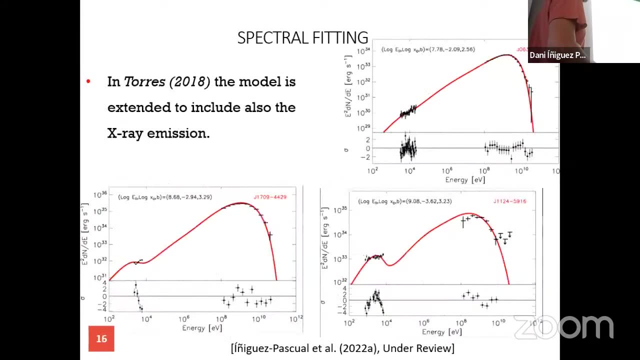 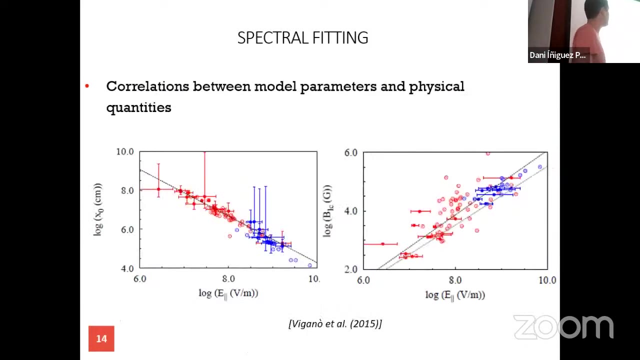 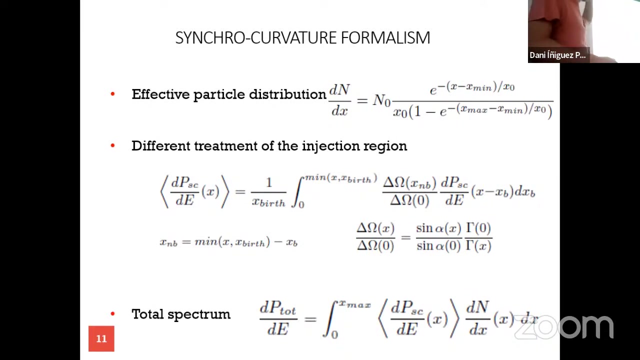 for what I would use. But why do you have the Netflix, the cable, the structure on the industry? because this is a consequence of this distribution. So the recipe parameters found for this zero are very small, so we use that. more weight is given to the inner part of the algorithm.